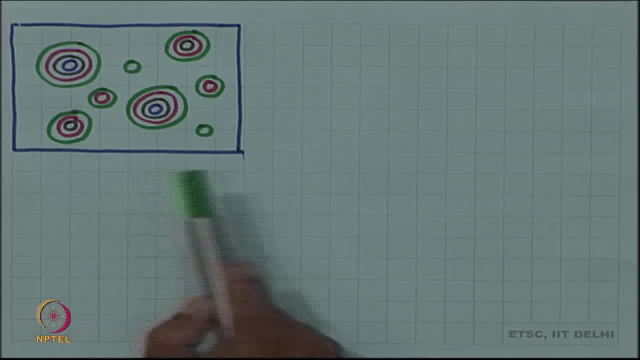 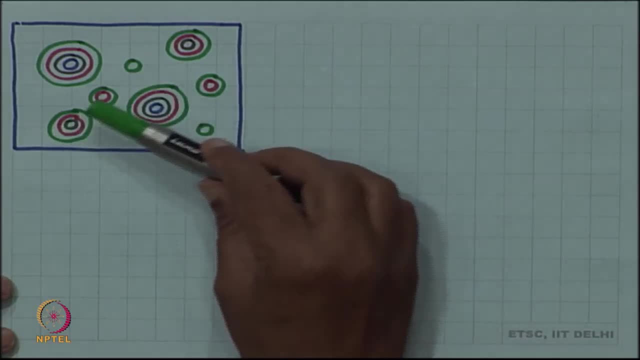 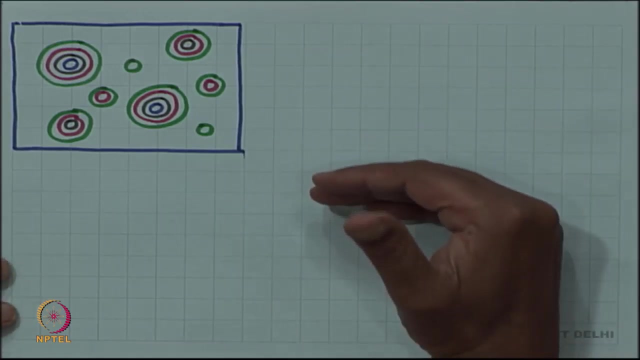 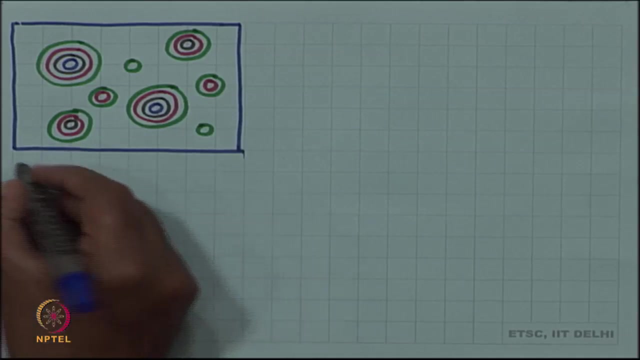 So one can see that gradually, with this process of nucleation and growth, New nuclei are forming and already existing particles are growing. So the overall transformation rate will depend upon both the nucleation rate and the growth rate. So let us define nucleation rate. 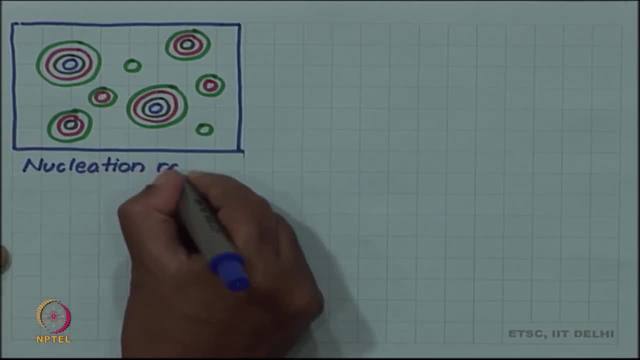 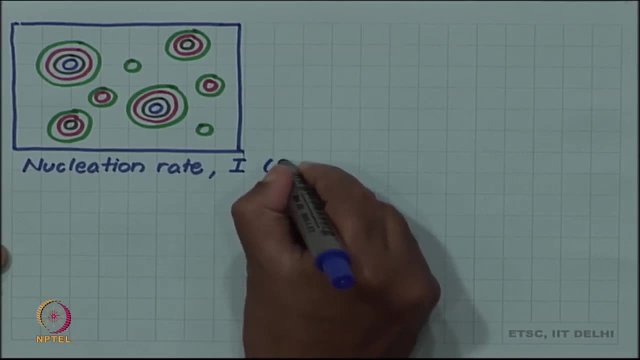 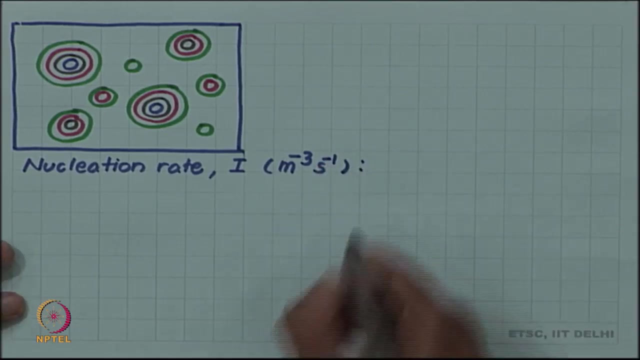 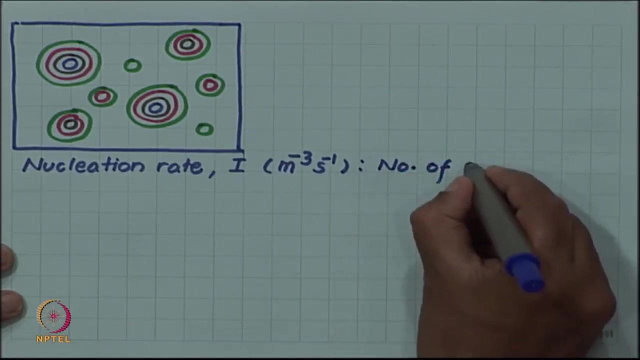 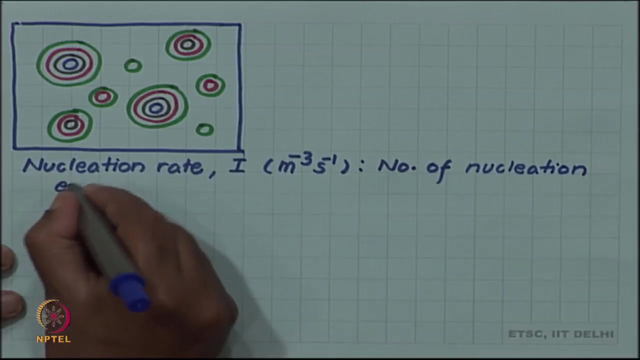 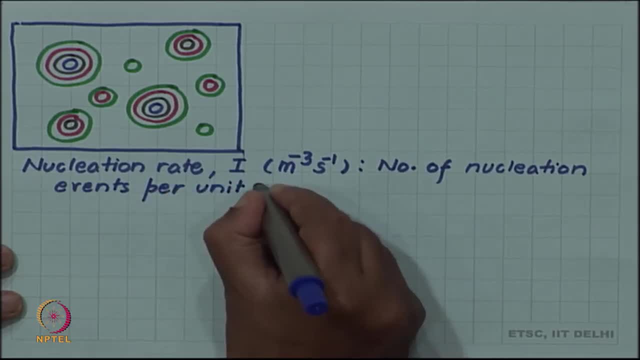 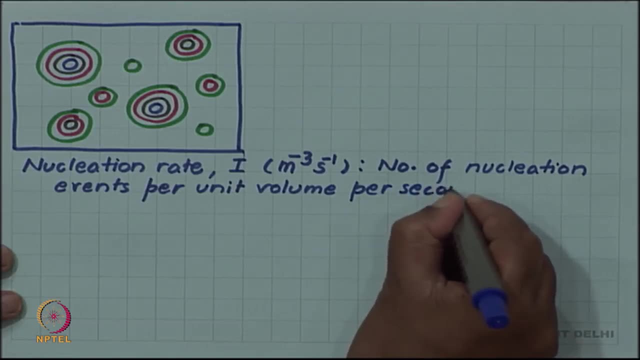 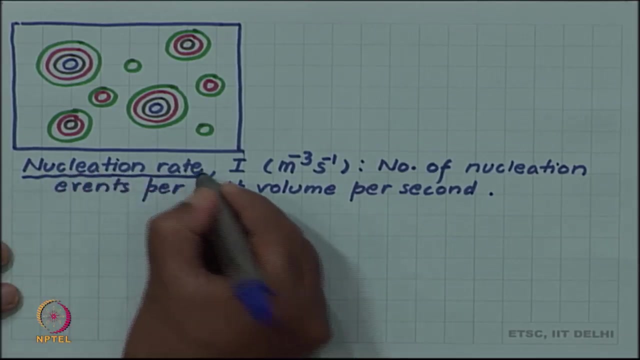 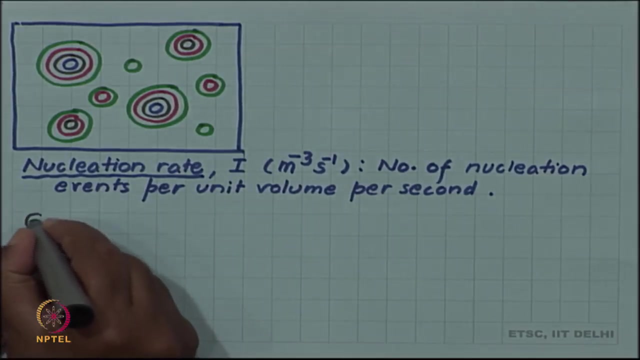 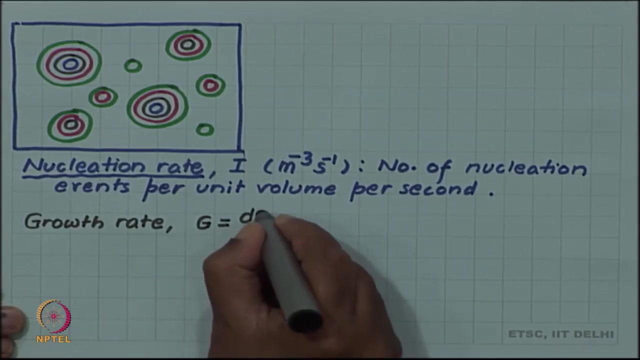 Per unit growth rate. volume per second. So that will be the nucleation rate. then we also have the growth rate. we give the symbol g. we can also call it dr by dt, where r is the particle size, So the units will be meters per second. 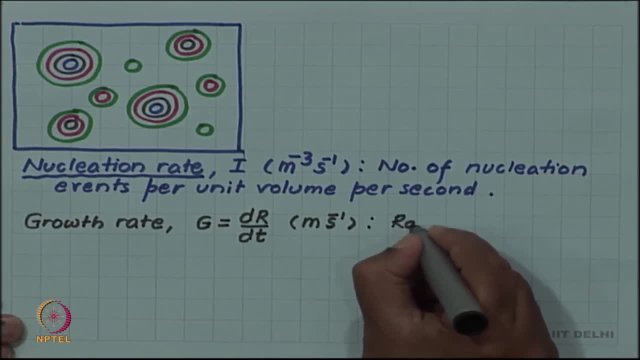 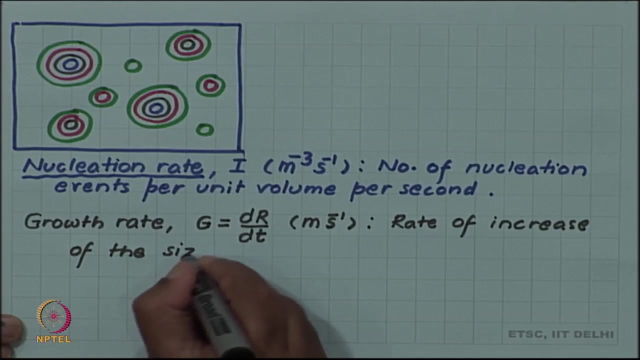 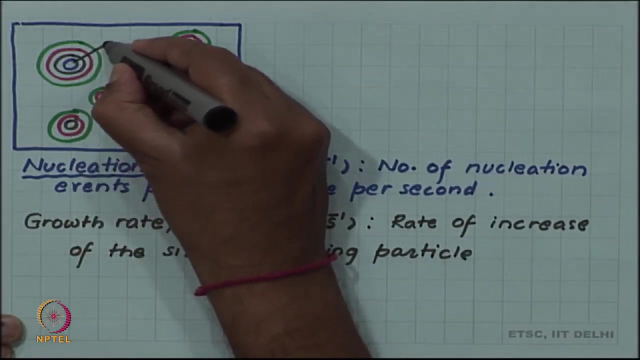 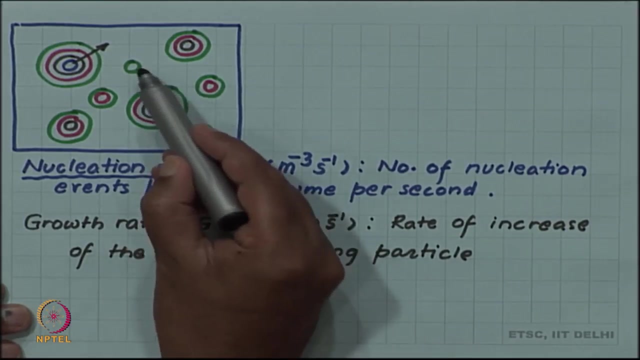 So this will be rate volume per second. So this is the rate of increase of the size of the particle. so that is at what rate this interface is moving. So that will be the growth rate. the nucleation rate will be at what rate new particles are.